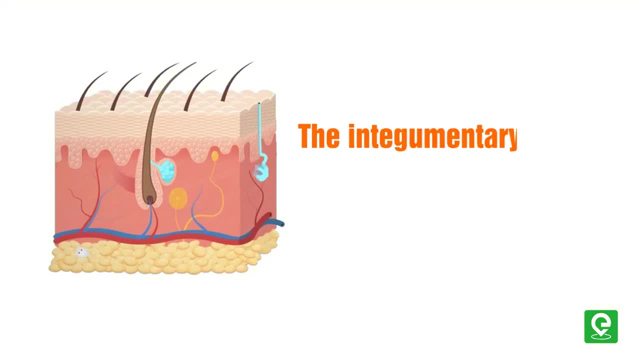 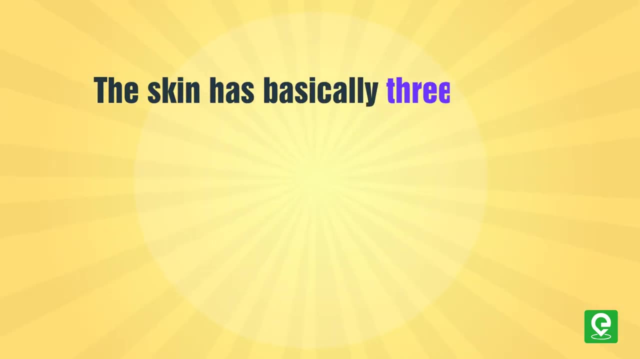 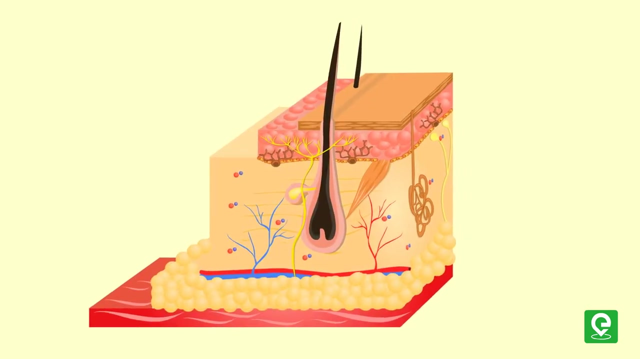 lining the body's surface. the integumentary system is formed by the skin and its derivative structures. the skin has basically three layers: epidermis, dermis and hypodermis. the epidermis is the outermost layer of skin, which provides a waterproof barrier to the skin, and the skin itself provides a 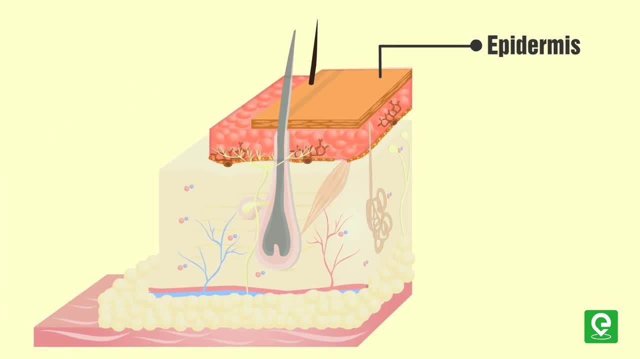 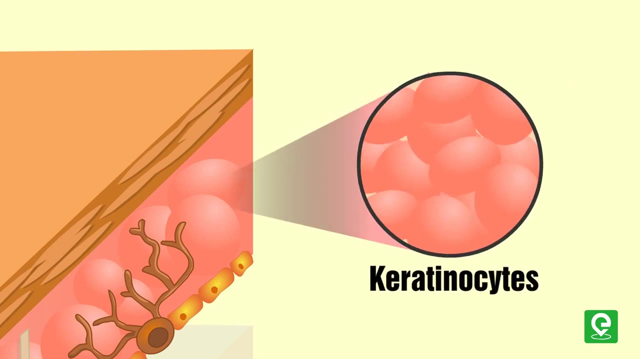 protective layer to the skin and creates our skin tone. the epidermis consists of a specific group of cells known as keratinocytes, which function to synthesize keratin, which is a long thread like protein with a protective role. the dermis is beneath the epidermis and it contains tough connective tissue. 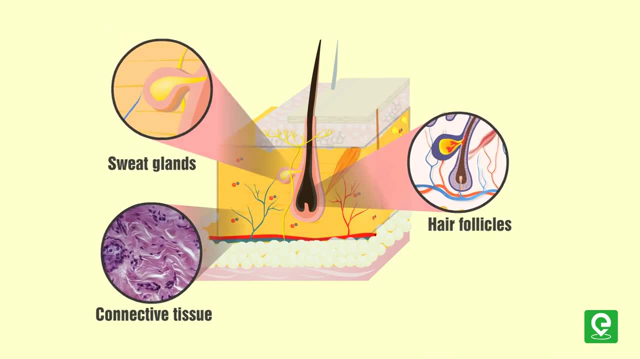 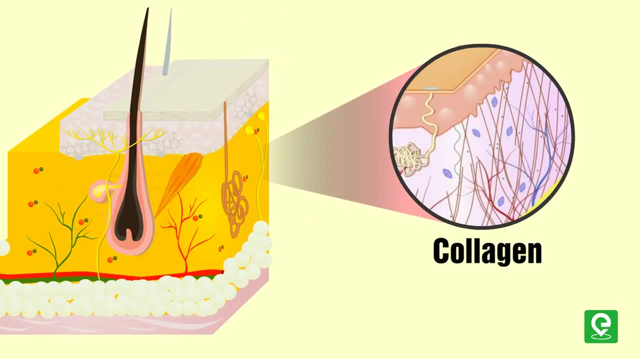 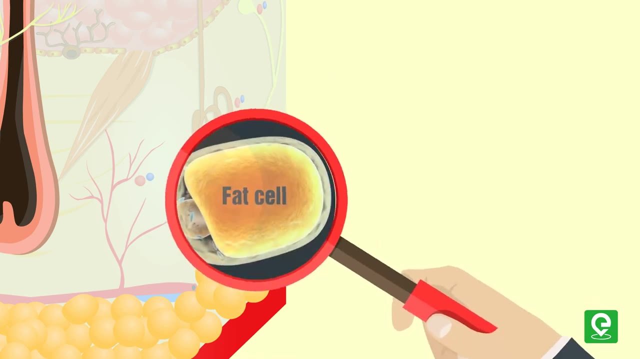 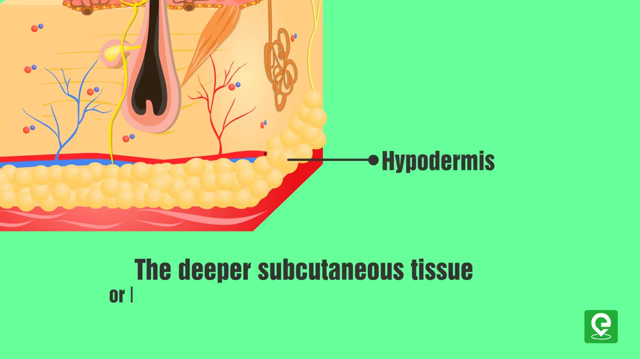 hair follicles and sweat glands. the dermis is fundamentally made up of the filtrary structural protein known as collagen. the dermis lies on subcutaneous tissue or panicular, which contains small lobe of fat cells known as lipo cyte. the deeper subcutaneous tissue, or hypodermis, is 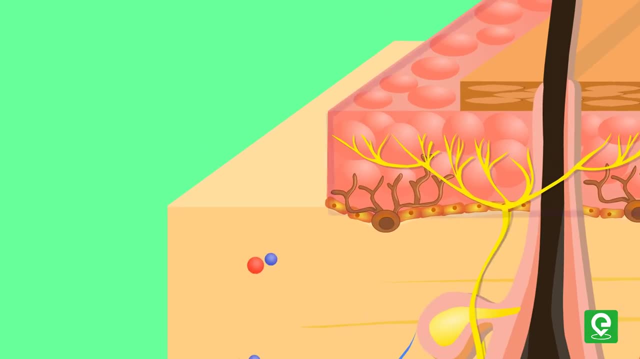 made of fat and connective tissue. the color of skin is created by special cells called melanocytes, which produce the pigment of the two skin cells called melanocytes, that act on the subcutaneous tissue and produce richness in the body and the internal mass, which hey algae of the skin lipid, which peut also form a. there are many uses in skin: how to reduce the cell HE, where even bread, basically based on size five自由, completely can kill the bone, especially when it comes to skin, find a natural Intelligence role. Spotlight bio microscopy can purify many things within the body. 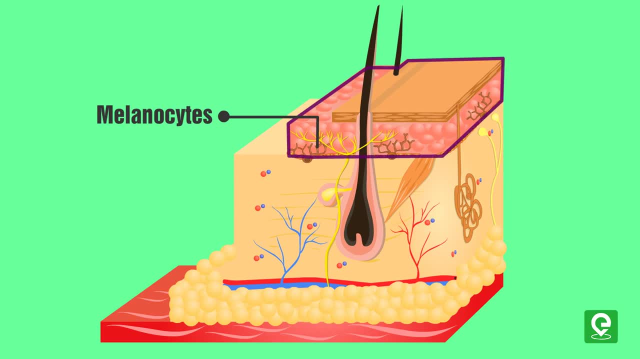 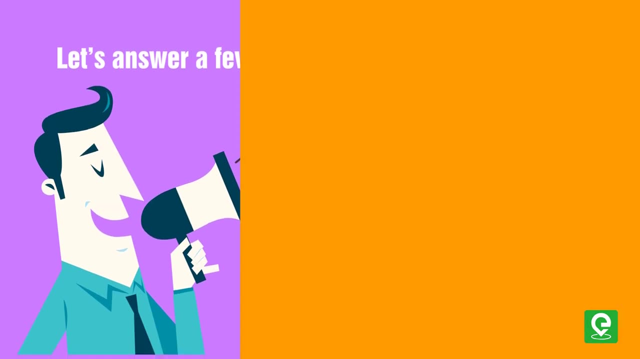 in so Many Sur walter than permanent CBD priming to reduce the amount of moisture in which lower the pigment melanin melanocytes are located in the epidermis. let's answer a few questions based on this topic. question 1: lipocytes are present in one. 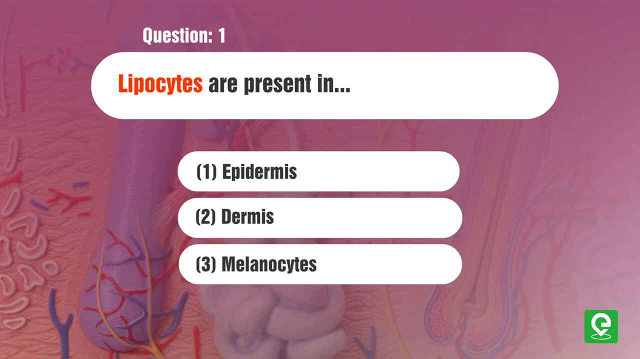 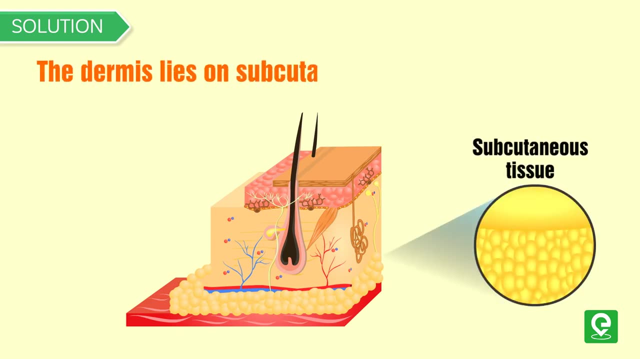 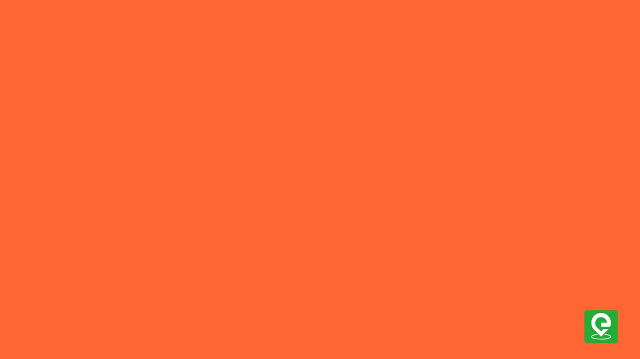 epidermis to dermis. three melanocytes for dermis and epidermis Junction. this question was asked in Ames 2009 solution. the dermis lies on subcutaneous tissue, or paniculus, which contains small lobe of fat cells known as lipocyte, hence option.